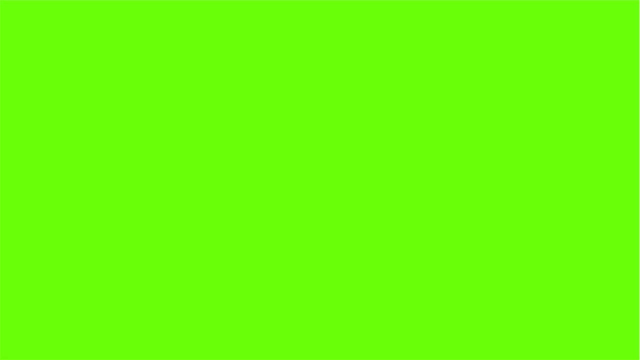 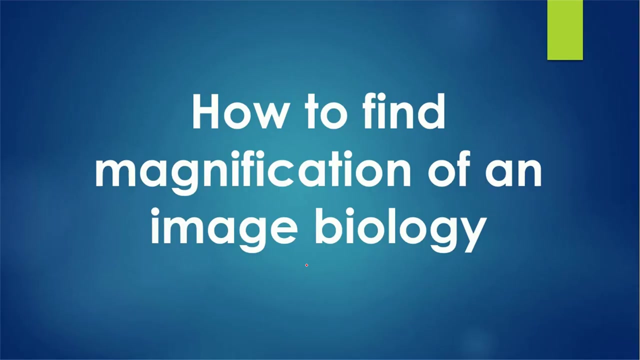 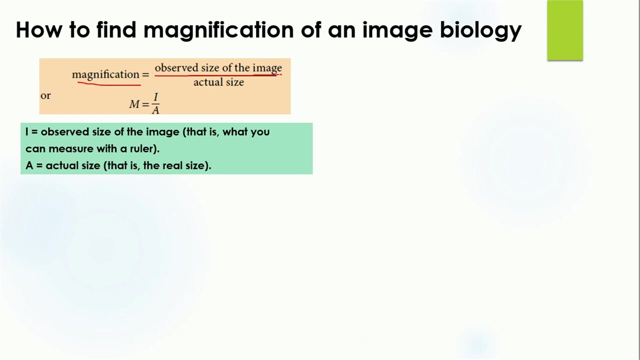 Hey learners, welcome to Amit Coaching and I'm your teacher, Dr Anand. Today we are going to study about how to find the magnification of an image. in biology, The formula for the magnification is: magnification is equal to observed size of the image divided by actual size. It's represented by 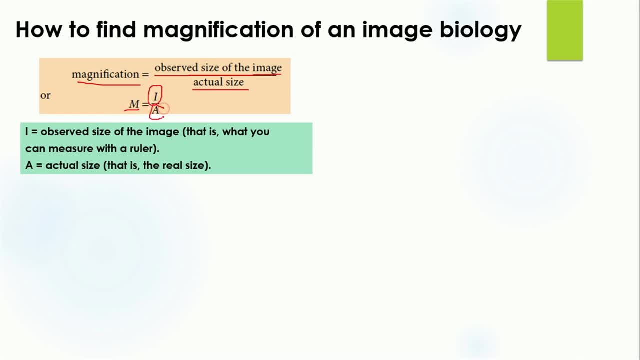 m is equal to i divided by a. Here, the i is the observed size of the image, and this is the size of the image that you are going to measure with your ruler, While the a is the actual size, that is the real size of that image. We can further clarify our this concept by using an example. 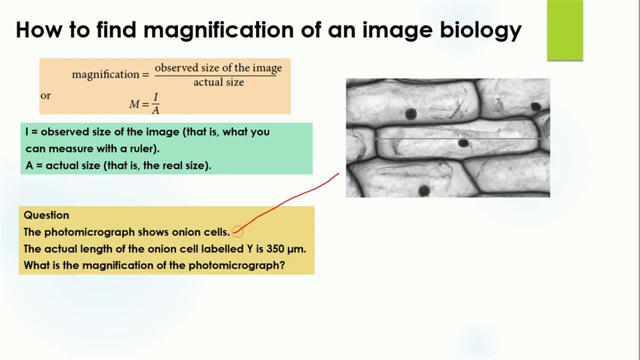 The photomicrograph shows an onion cell, this one here. The actual length of onion cell labeled y is 350 micrometer. Here we can see that this here is the y cell and its actual length is 350 micrometer. What is the magnification of the? 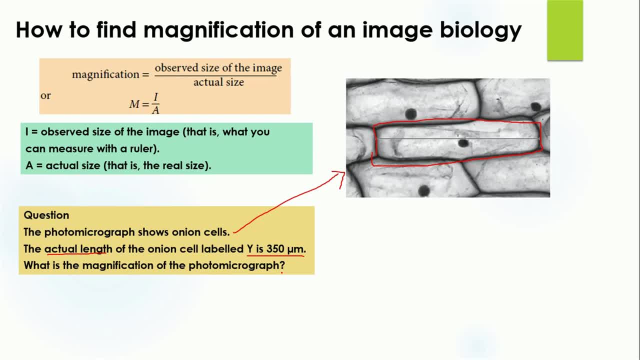 photomicrograph. So how we are going to solve it In step one, we are going to measure the y with the ruler. So from this point, we are going to measure the y with the ruler. So from this point, we are going to measure the y with the ruler. So from this point to this point, you are going to measure. 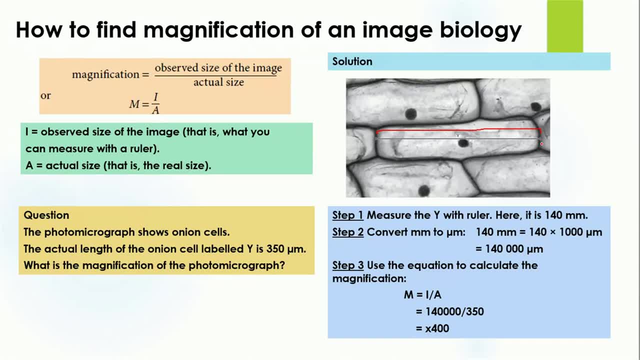 this straight line with the help of your ruler. Your ruler is going to give you the value in millimeter, and in this case, the value is 140 millimeter. Whenever you are doing the magnification calculations, always convert your values into micrometer. Why to convert it into micrometer? 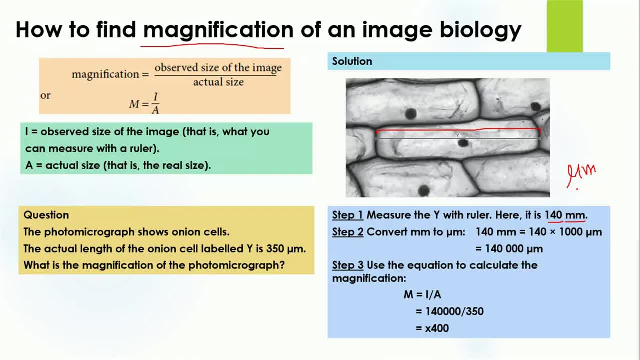 Because the cells are very small in size, So the cells are very small in size, So the cells are very small in size, So it's better to use micrometer. So in step two we will convert the millimeter into micrometer and for this we are going to multiply 140 millimeter with 1000.. So we are getting this value.